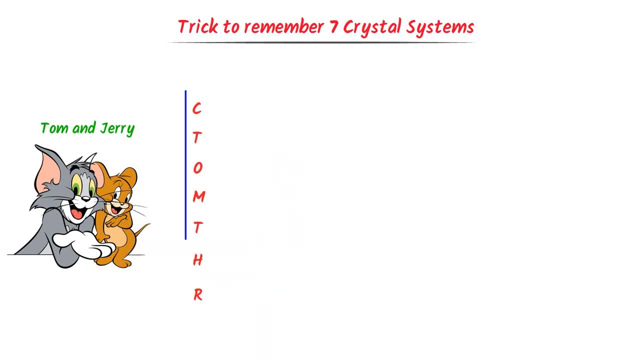 see Tom there. Let me repeat it: See Tom there. This C stands for cubic, This T stands for tetragonal, This O stands for octahedral, This M stands for monoclinic, This T stands for triclinic, This H stands for hexagonal And this R stands for rhombohedral. 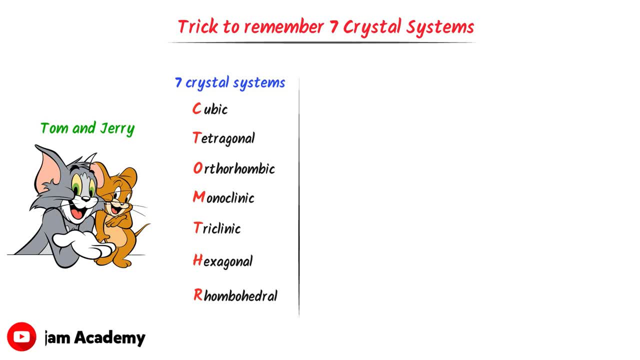 These are the seven crystal systems. Now, what about their respective edge lengths? Well, the first and the last one have the same edge lengths: A equals B, B equals C. A equals B, B equals C. The second and last one have the same edge lengths. 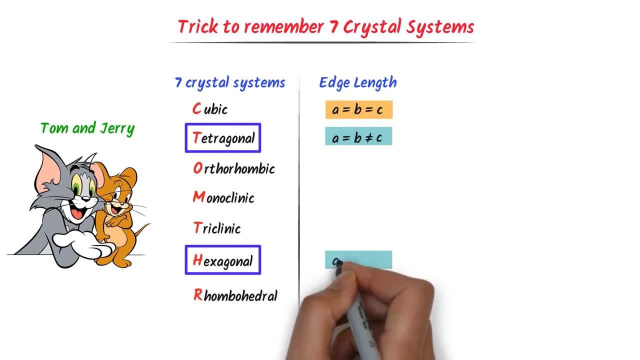 A equals B, But B doesn't equal C. A equals B, But B doesn't equal C. These remaining three systems have the same edge lengths. A is not equal to B. B is not equal to C. A is not equal to B, B is not equal to C. A is not equal to B. B is not equal to C. 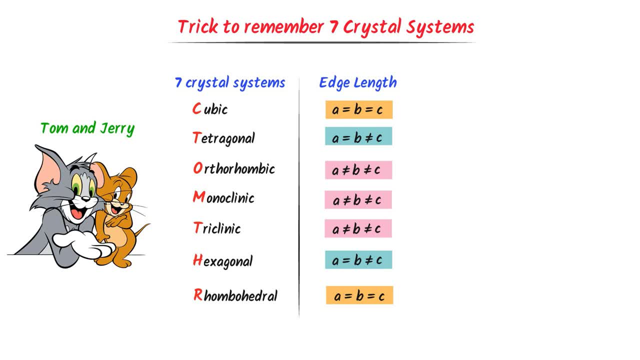 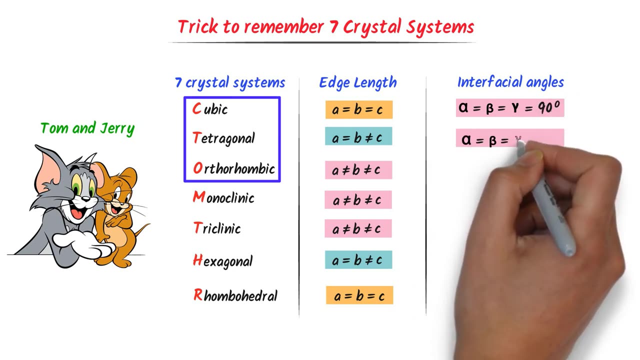 Hence, these are the lengths of these seven crystal systems. Now, what about their respective interfacial angles? Well, the first three have the same angles: Alpha equals beta, Beta equals gamma, Alpha equals beta, Beta equals gamma, Alpha equals beta, Beta equals gamma. 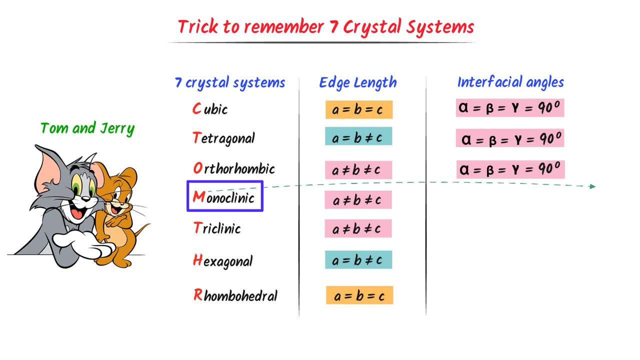 Now there is M and this monoclinic. If I rotate this M 90 degree clockwise and I draw here line, it is like B, This beta and 90 degree reminds me. beta is not equal to 90 degree. The remaining two angles are: 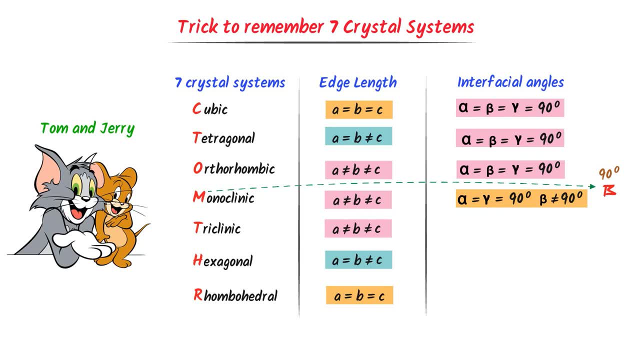 alpha is equal to gamma. Gamma is equal to 90 degree. In case of triclinic, there is a word, tri. This tri reminds me that three angles of the triclinic are not equal. Alpha is not equal to beta. 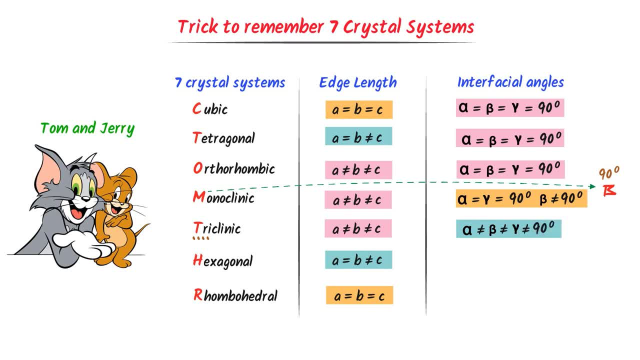 Beta is not equal to gamma. In case of hexagonal, I write: alpha is equal to beta, Beta is equal to 90 degree, Alpha is equal to beta, Beta is equal to 90 degree. Then I write: gamma is equal to and gamma is not equal to. 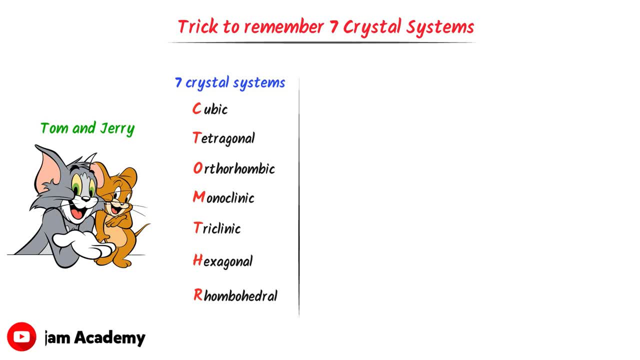 These are the seven crystal systems. Now, what about their respective edge lengths? Well, the first and the last one have the same edge lengths: A equals B, B equals C. A equals B, B equals C. The second and last one have the same edge lengths. 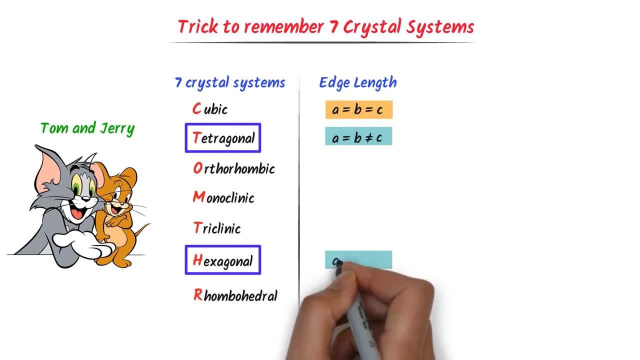 A equals B, But B doesn't equal C. A equals B, But B doesn't equal C. These remaining three systems have the same edge lengths. A is not equal to B. B is not equal to C. A is not equal to B, B is not equal to C. A is not equal to B. B is not equal to C. 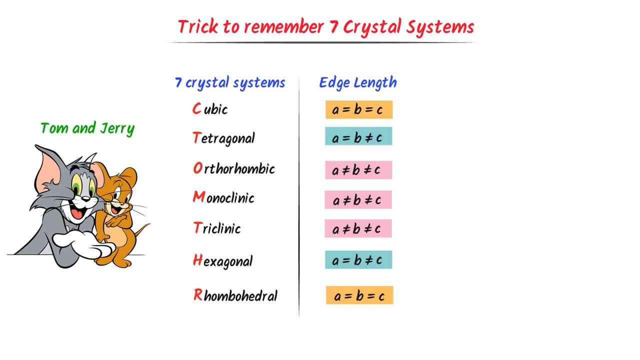 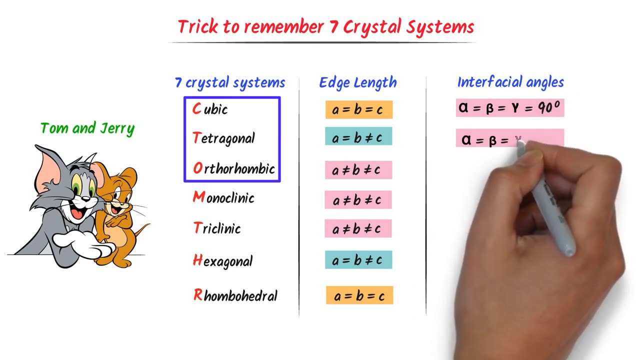 Hence, these are the lengths of these seven crystal systems. Now, what about their respective interfecial angles? Well, the first three have the same angles: Alpha equals Beta, Beta equals Gamma, Alpha equals Beta, Beta equals Gamma, Alpha equals Beta, Beta equals Gamma. 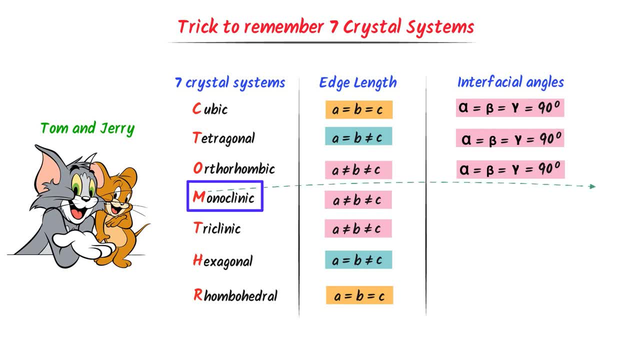 Now there is M and this monoclinic. If I rotate this M ninety degree clockwise and I draw here line, It is like beta. This beta and 90 degree reminds me beta is not equal to 90 degree. The remaining two angles are: alpha is equal to gamma, gamma is equal to 90 degree. 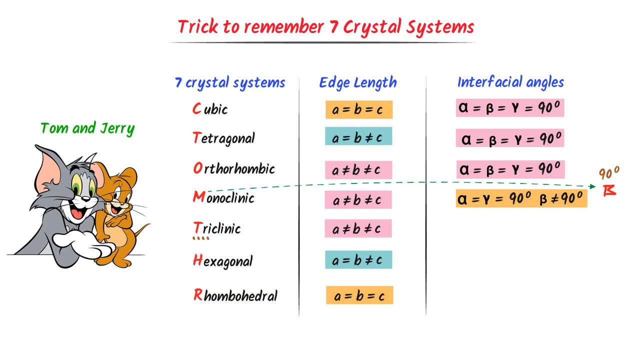 In case of triclinic, there is a word tri. This tri reminds me that three angles of the triclinic are not equal. Alpha is not equal to beta, beta is not equal to gamma. In case of hexagonal, I write: alpha is equal to beta, beta is equal to 90 degree. 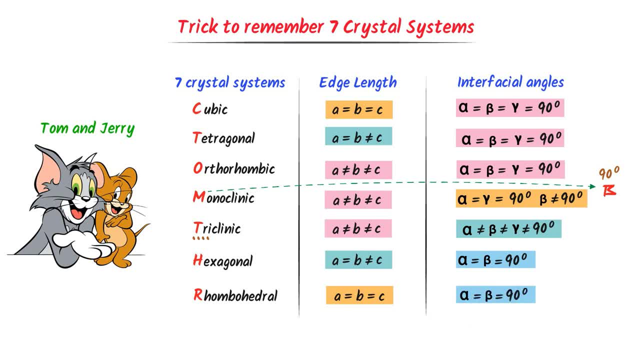 Alpha is equal to beta, beta is equal to 90 degree. Then I write gamma is equal to and gamma is not equal to. I write 120 degree and 90 degree. So everything is just boomed. Therefore, using this trick, we can super fastly learn and remember seven crystal systems. 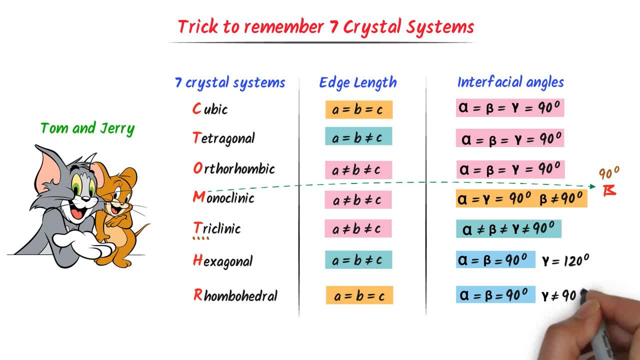 I write 120 degree and 90 degree, So everything is just boomed. Therefore, using this tric, we can superfastly learn and remember seven crystal systems. Now let me teach you that. how can we use these information to crack any question? 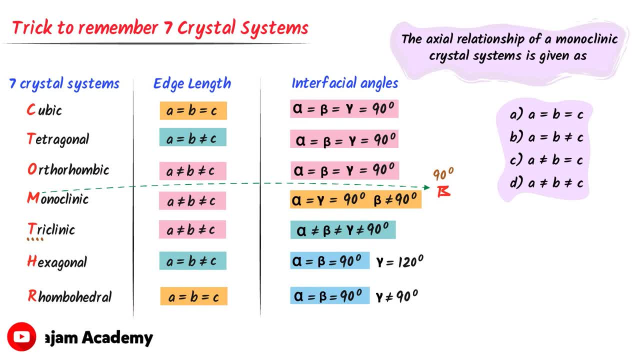 For example. consider these mcqs. The axial relationship of a monoclinic crystal system is: can you guess the answer? Well, according to this information, the edge length of a monoclinic system is: A is not equal to B. 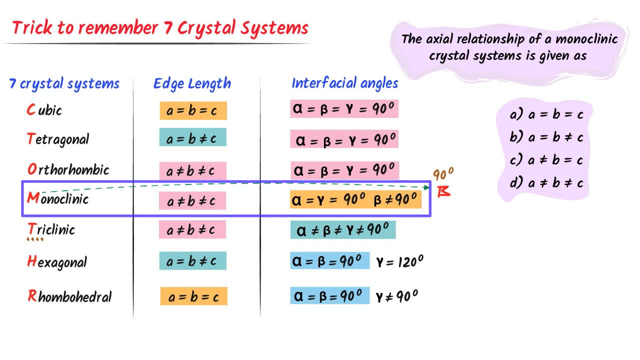 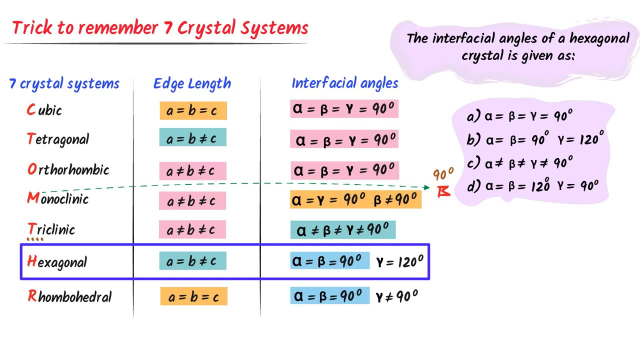 equal to B. B is not equal to C, So the correct option is D. Secondly, consider this: MCQs, The interfacial angles of a hexagonal crystal systems are given by well, according to this information, the correct option is B. Alpha is equal to. 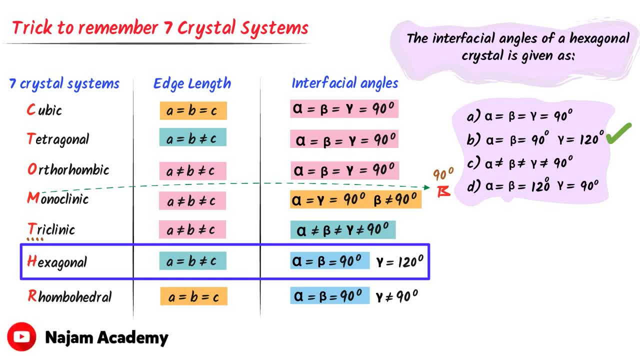 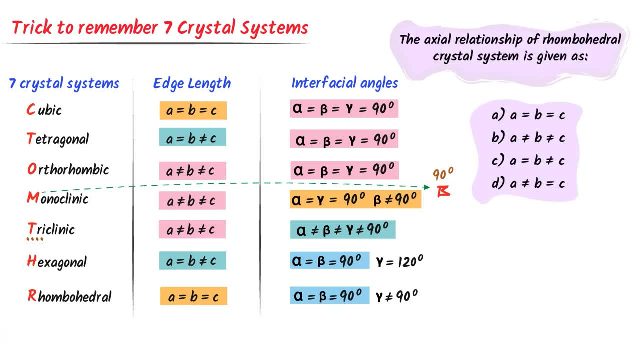 beta. beta is equal to 90 degree, but gamma is equal to 120 degree. Thirdly, consider this MCQs. The axial relationship of a rhombohedral crystal system is given as, according to this information, the correct option is A. A is equal to B, B is equal to C. Fourthly, consider this: MCQs, The 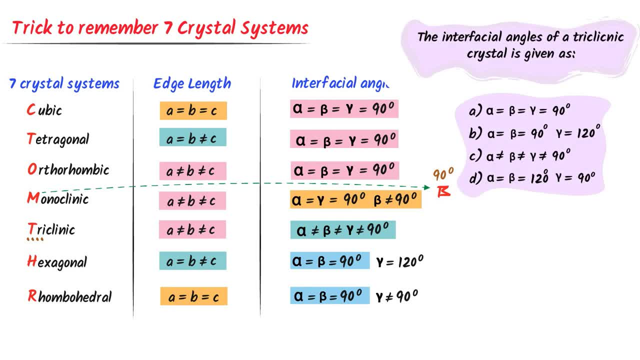 interfacial angles of a hexagonal crystal system are given by. well, according to, of a triclinic crystal system are given by. according to this information, alpha is not equal to beta, beta is not equal to gamma, and they all are not equal to 90 degree. Thus, 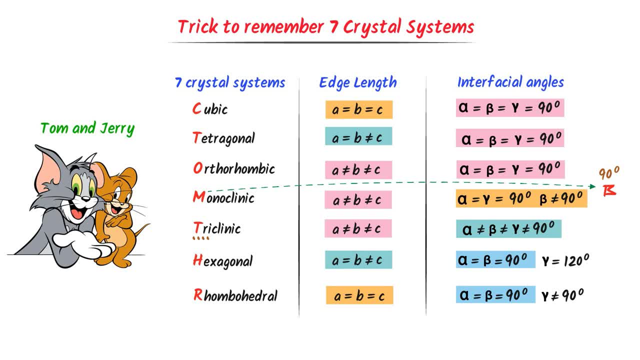 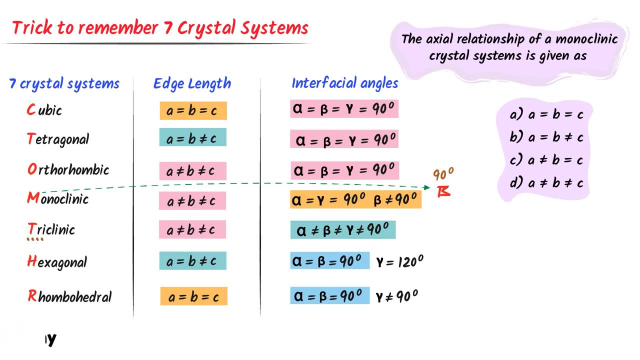 Now let me teach you that. how can we use this information to crack any question? For example, consider this: MCQs. The axial relationship of a monoclinic crystal system is: can you guess the answer? Well, according to this, 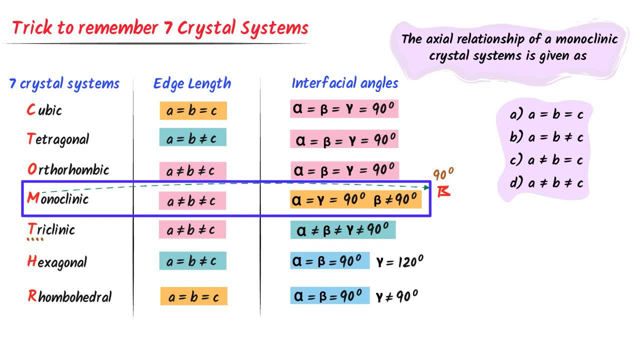 information. the edge length of a monoclinic system is: A is not equal to B, B is not equal to C, So the correct option is D. Secondly, consider this MCQs: The interfacial angles of a hexagonal crystal systems are given by: 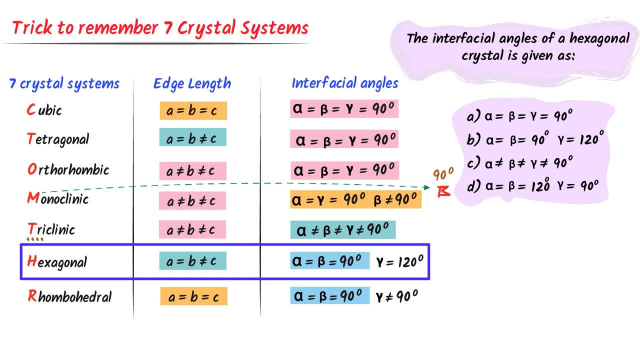 well, according to this information, the correct option is B. Alpha is equal to beta, Beta is equal to 90 degree, but gamma is equal to 120 degree. Thirdly, consider this MCQs. The axial relationship of a rhombohedral crystal system is given as: 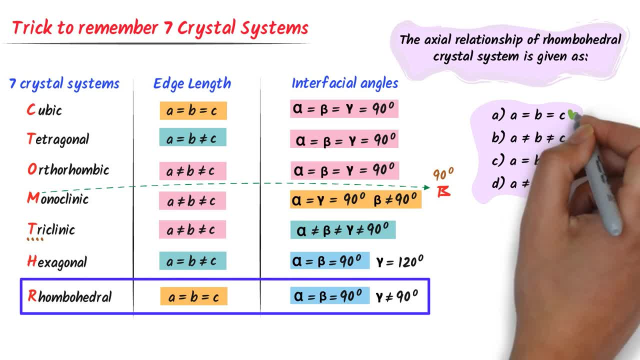 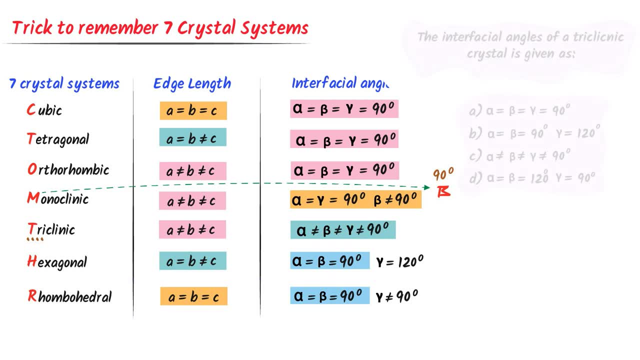 according to this information, the correct option is A. A is equal to B, B is equal to C. Fourthly, consider this MCQs: The interfacial angles of a triangle system are given by. well, according to this information, the correct option is A. 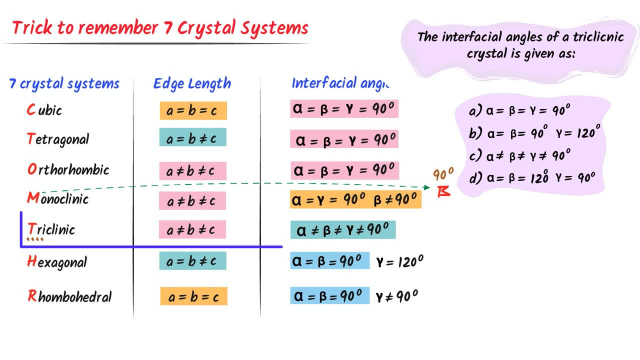 A is equal to B. B is equal to C. The interfacial angles of a triclinic crystal systems are given by well. according to this information, the correct option is B. Alpha is not equal to beta. Beta is not equal to gamma. 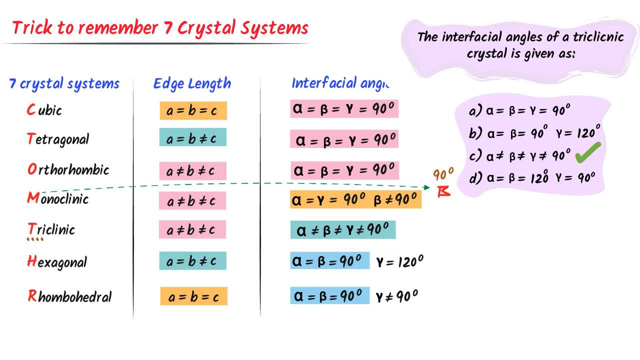 And they all are not equal to 90 degree. Thus, using this trick, we can easily remember the seven crystal systems. Also, we can crack any exam question using this super easy trick. 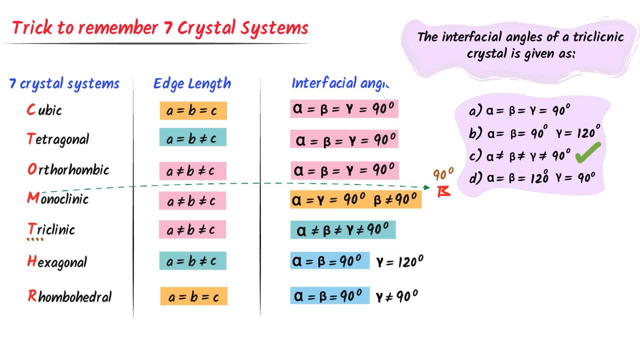 using this trick, we can easily remember the seven crystal systems. Also, we can crack any exam question using this super easy trick.